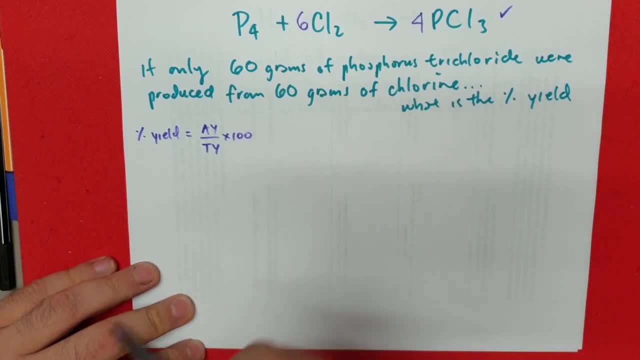 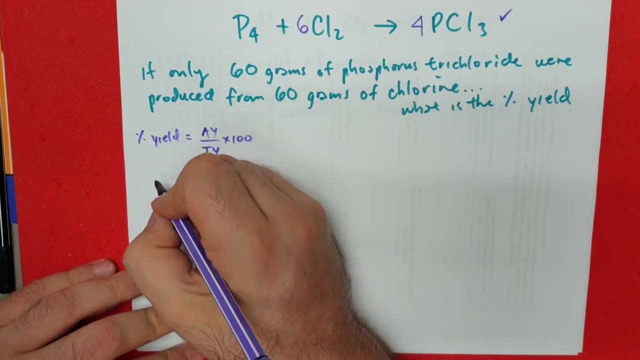 60 grams of chlorine. what is the percent yield? so we already have the actual yield, because it says: if only 60 grams of phosphorus trichloride were produced. so we're just going to plug it in right here and my actual yield is 60 grams of phosphorus trichloride, meaning that we want to calculate the. 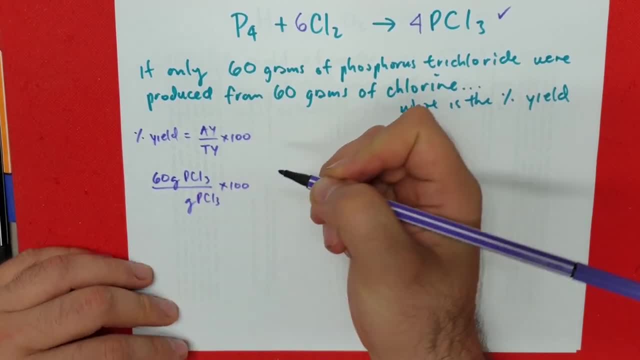 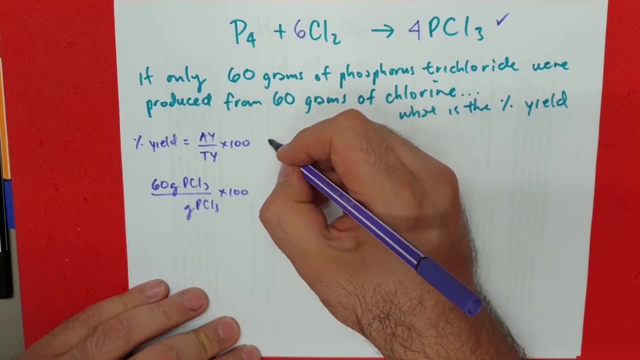 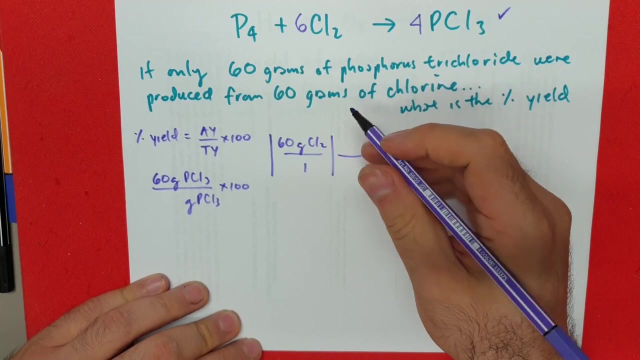 theoretical yield of phosphorus trichloride and multiply it times 100. so for that i'm going to set up a mass mass problem with the 60 grams of chlorine. so 60 grams of chlorine over one. then i add the molar mass of chlorine, which is 70.9 grams of chlorine for every mole of chlorine. 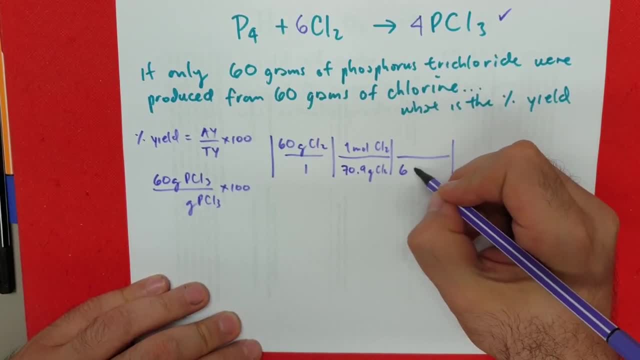 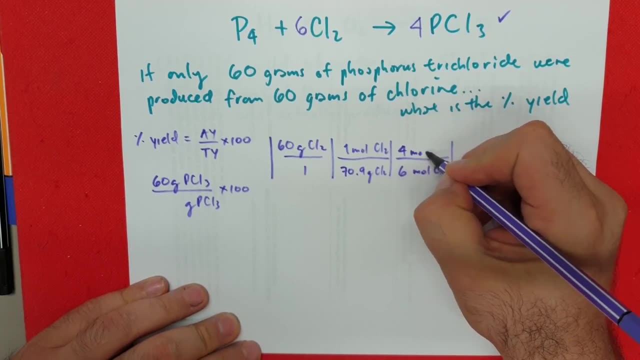 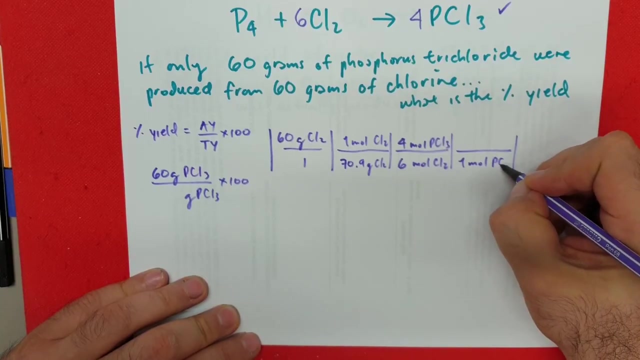 next up is six moles of chlorine. why six? because that comes from the balance equation and i want to convert to moles of phosphorus trichloride. so phosphorus trichloride goes here, and my last step is to calculate the molar mass of phosphorus trichloride, which is 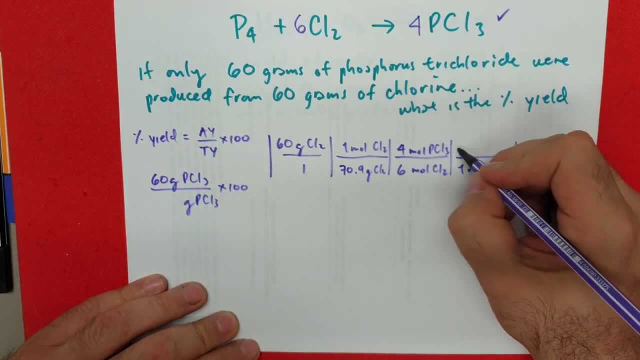 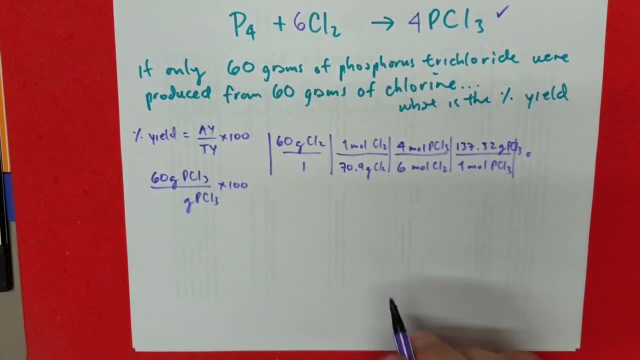 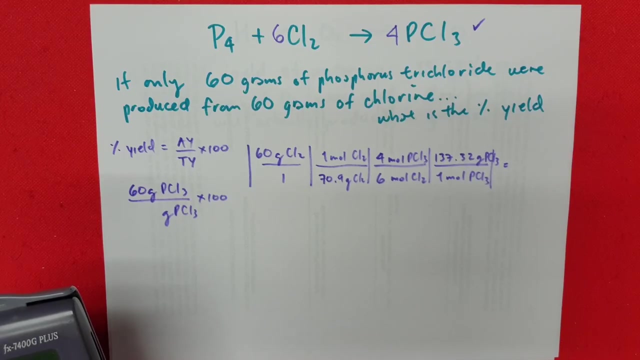 if I add up three atoms of chlorine and one of phosphorus, gives me 137.32 grams of phosphorus trichloride. So right now, with this number, what we did is we calculated the actual yield of chlorine 60 times, 4 times 137.32, divided by 70.9 times 6, and that gives me a grand total of rounded up. 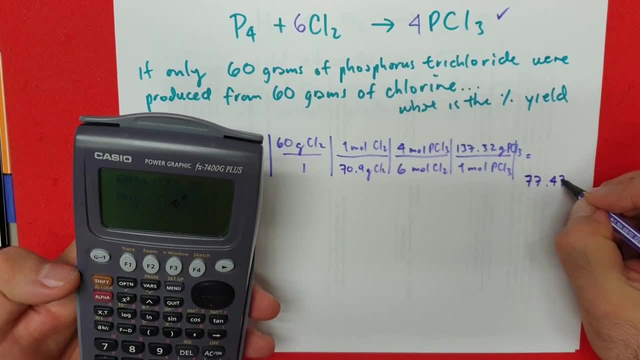 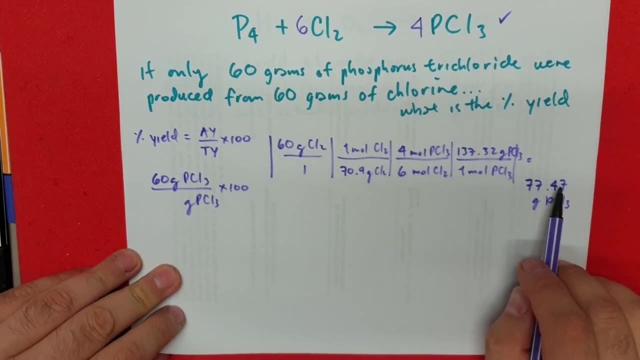 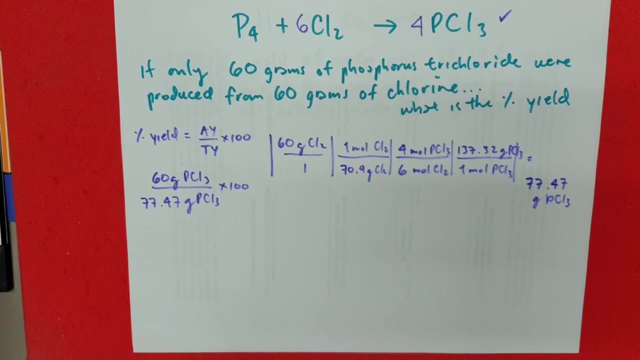 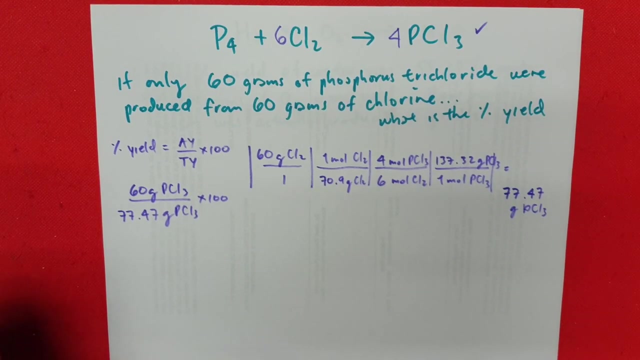 77.47 grams of phosphorus trichloride. So in this case this is my theoretical yield, and now I can just take this number and put it into the formula and write 77.47, and then it's just very simple math. I'm going to take 60 and divide it by 77.47 and then multiply it times 100, and 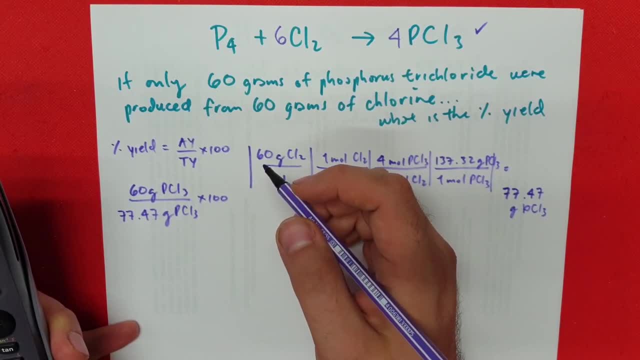 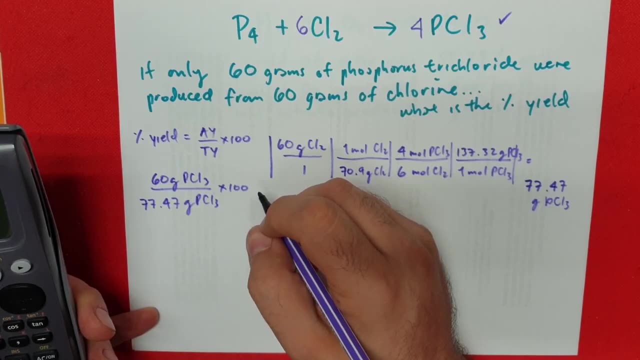 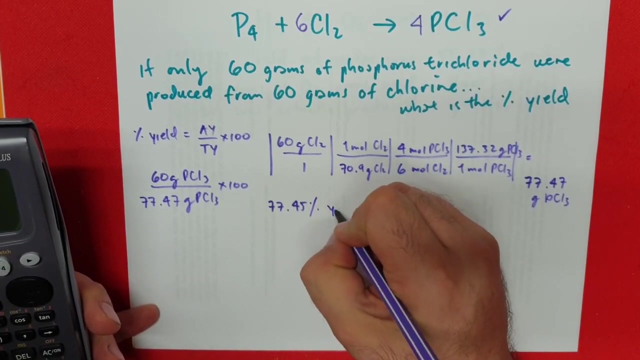 round it up and my percentage is very interesting because it gives me, if I did this right, oh so interesting- 77.45 percent yield of phosphorus trichloride. So in this case, I'm going to box it up and I'm going to write 77.47, and then I'm going to 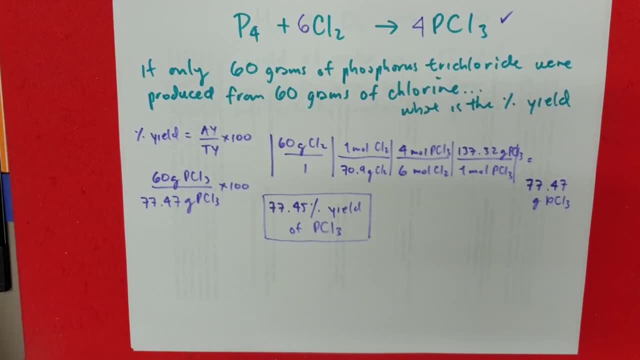 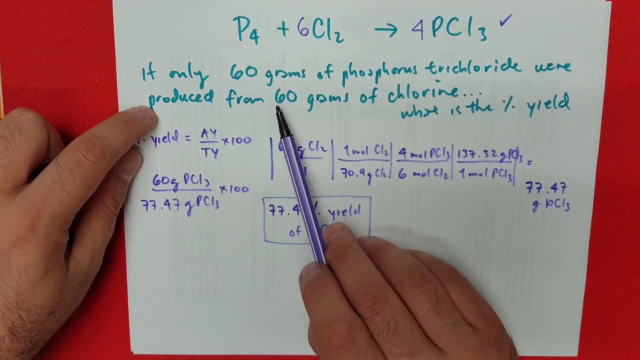 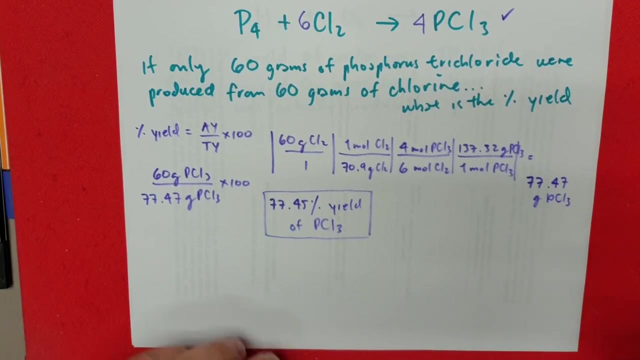 calculate it, because this is my final answer and it's very simple. So remember, we were given two pieces of information, an actual yield, and we were given one of the reactants so that we can calculate our theoretical yield, and then we multiply it by 100.. Now another example which 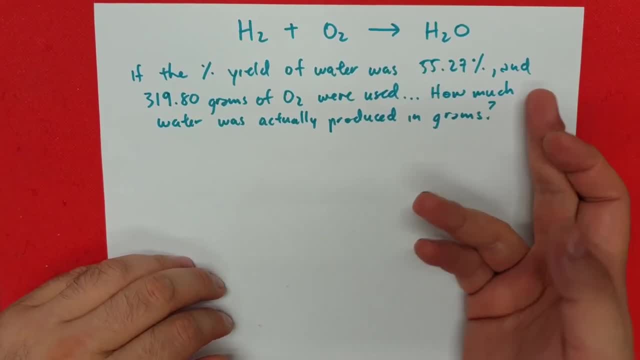 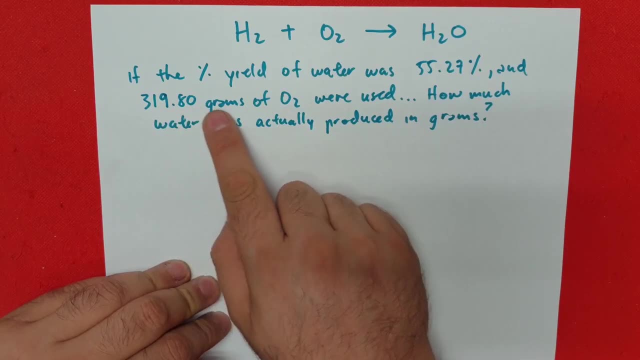 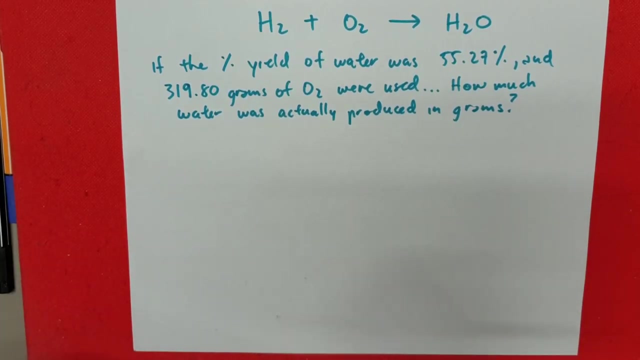 we can get is: we have this reaction, of course, and it says: if the percent yield of water was 55.27 and 319.80 grams of oxygen were used, how much water was actually produced in grams? So here let's take the vocabulary, and once again, we can chop up this problem in many different ways. The first: 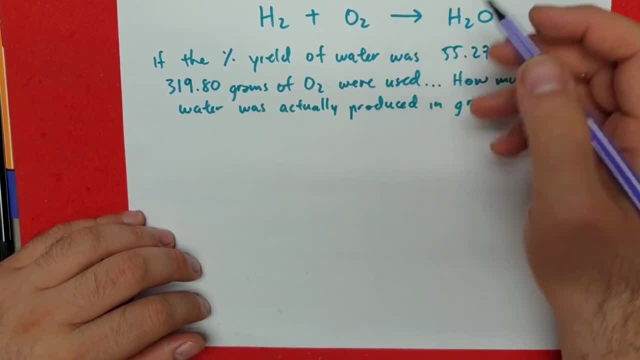 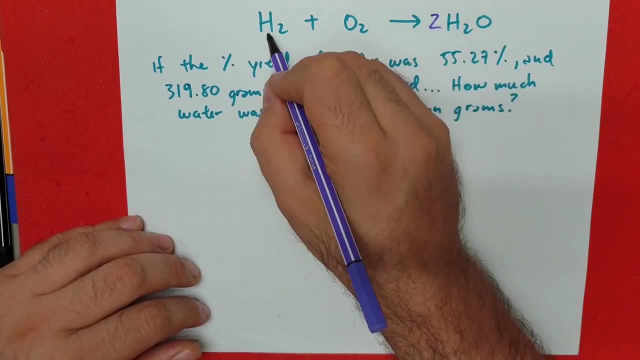 thing I'm going to do, though, is balance. just to make sure, is this balanced? it's not. I added two to balance the oxygen, but now hydrogen became four. on this side we have two. I'm going to add a two, and now we're balanced, So remember. 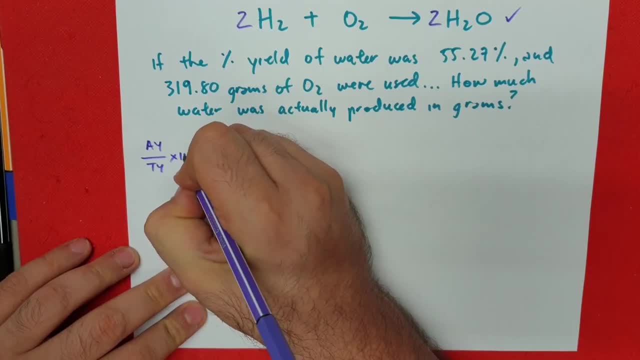 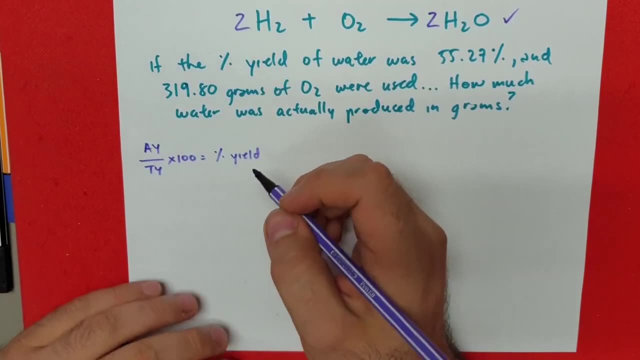 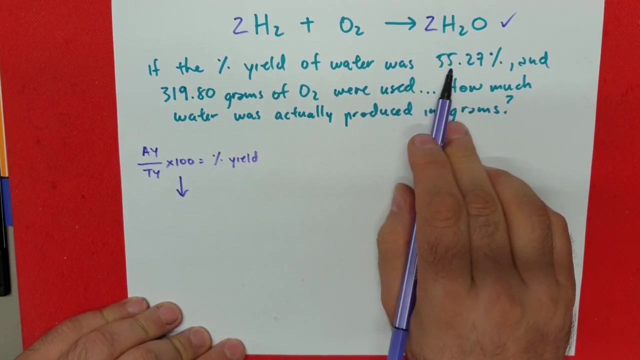 actually yield. divided by theoretical yield times 100 equals percent yield. So what I'm going to try to do here is I'm going to do the algebraic manipulation so that we're going to get our answer right away at the end. So what we're looking for is if the percent yield of water 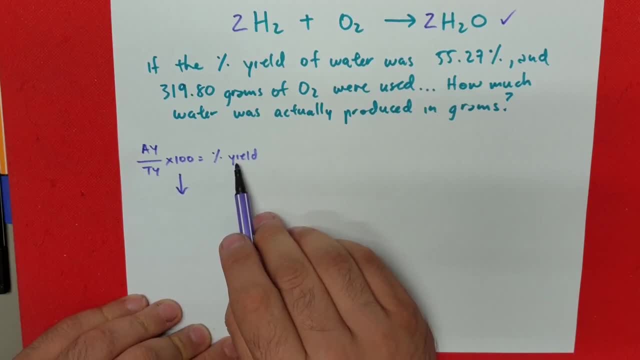 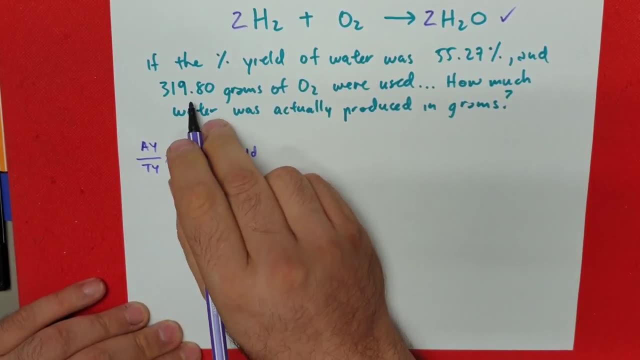 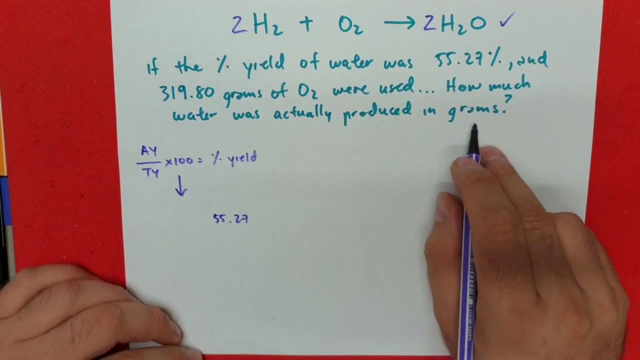 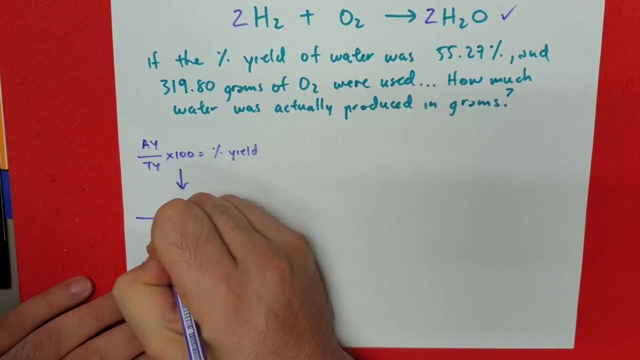 was 55.27, which we already have. let's just plug it right there, and it's 55.27 and 319.80 grams of water, of oxygen, were used. how much water was actually produced in grams? so we don't have all the pieces of information here, we only have the the. 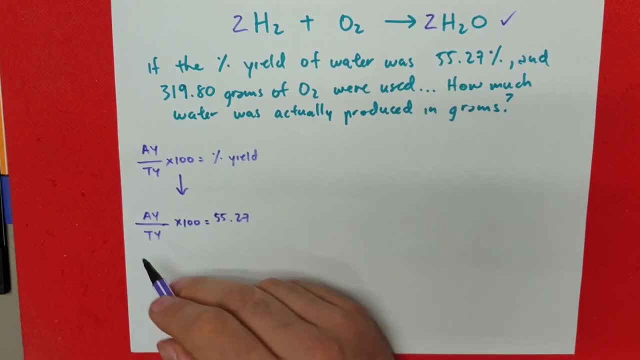 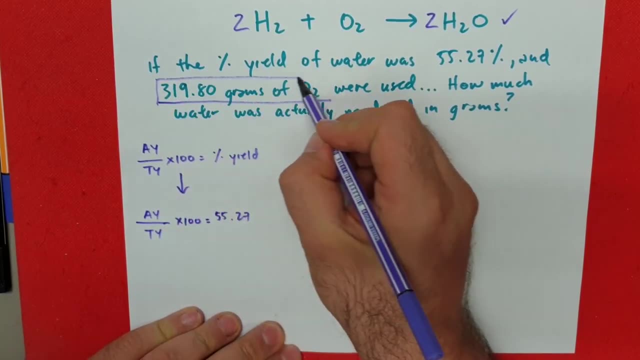 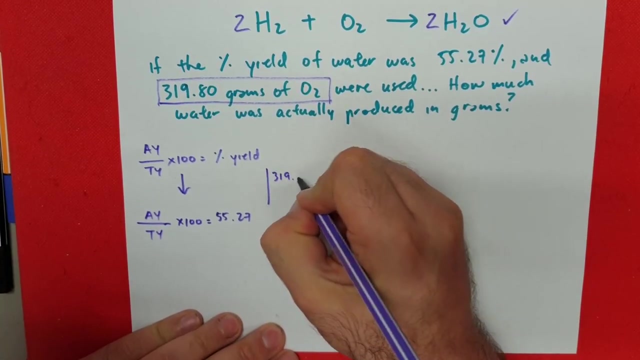 way to calculate theoretical yield. so, in order to get that theoretical yield over here, what do I need to do? I need to take this given, which is one of the reactants involved, and we're going to take a mass, mass problem and we're going to say 319. 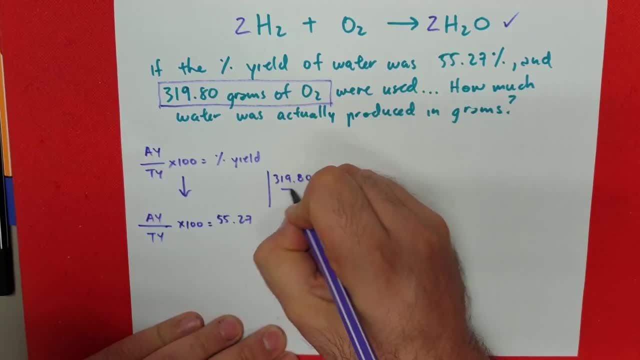 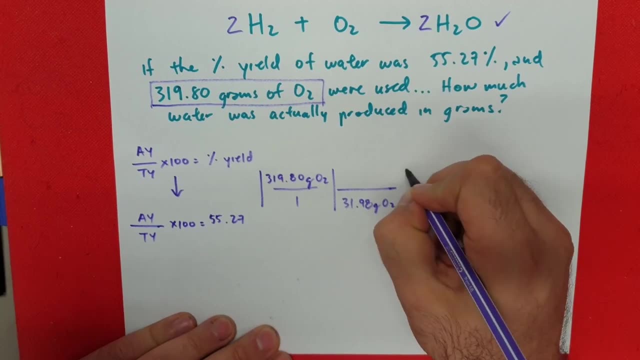 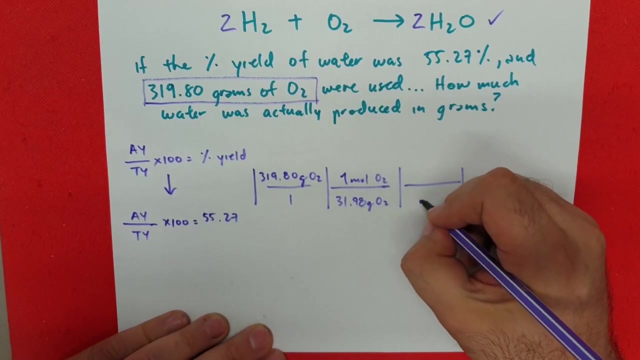 point 80 grams of oxygen over 1. the molar mass of diatomic oxygen is 31 point 98 grams of oxygen over 1 mole of oxygen. then we look at our chemical equation to convert to moles, moles of oxygen, and we want to know moles of water, which is 1. 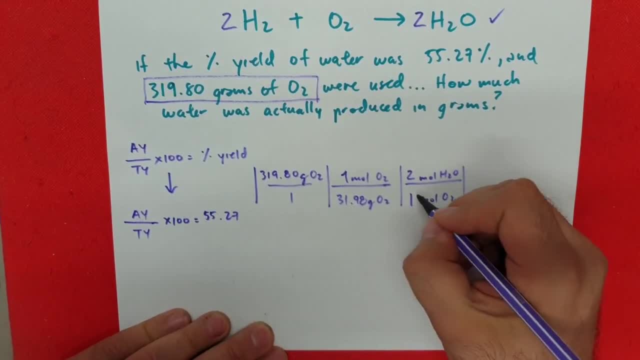 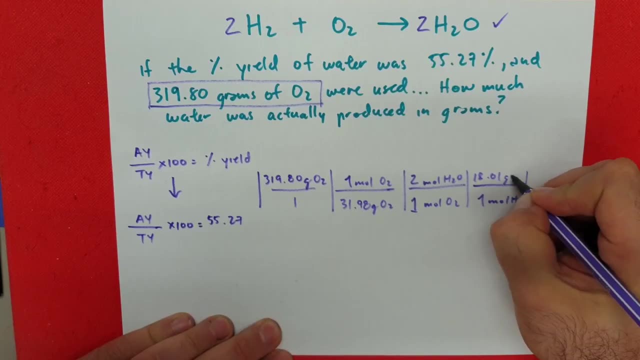 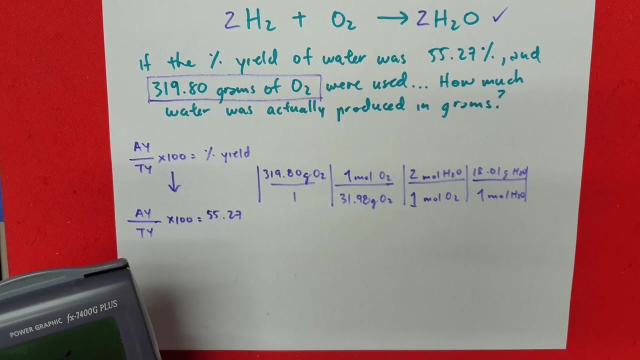 mole of oxygen for every two moles of water from our balance equation and, last but not least, the molar mass of water, which is 18.01 grams of water. so once we punch this into the calculator and after everything cancels out, we take 31, 319 point 80 times. 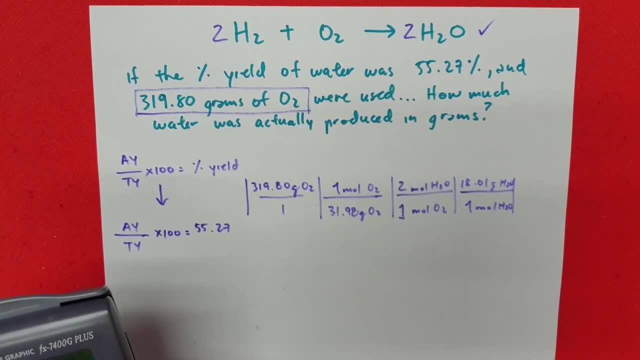 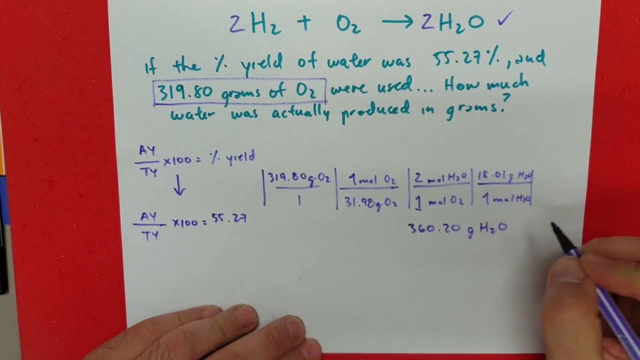 2 times 18.01 and we divided by 31 point 98, so this reaction should have given us a theoretically 360 point 20 grams of water. so this is equal to our theoretical yield. so now we have enough information, because a percent yield was given by the. 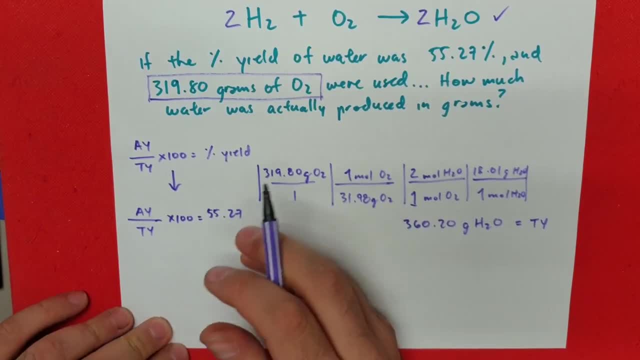 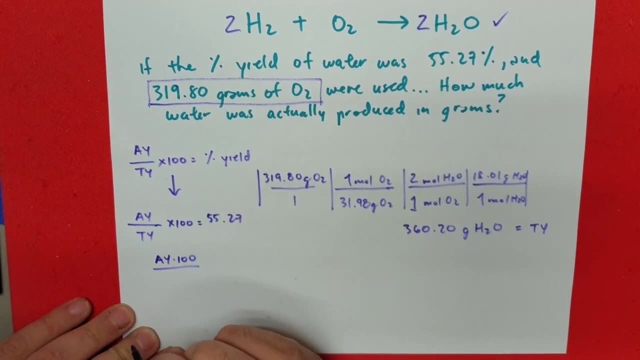 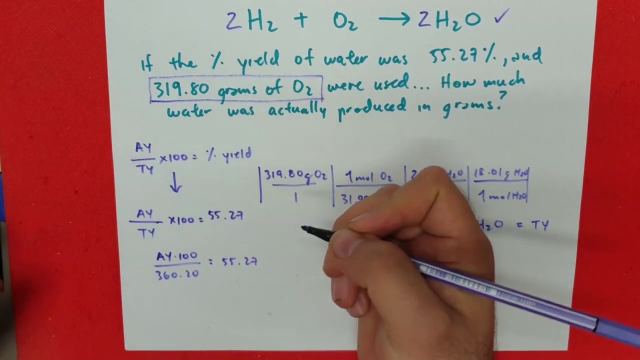 problem. we calculated the theoretical yield and now all we have to do is a little bit of algebra. so a Y times 100 divided by 360 point 20 is equal to 55.26. so I'm going to switch this 360 on the other side by multiplying. 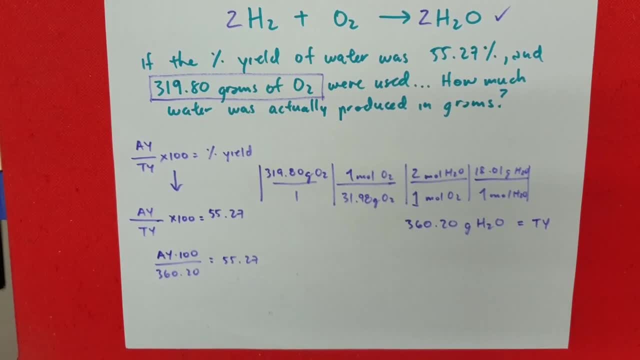 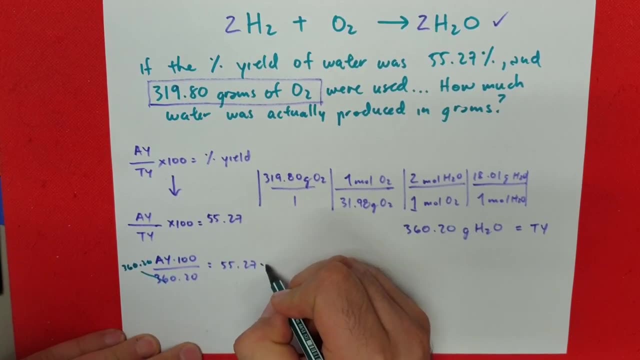 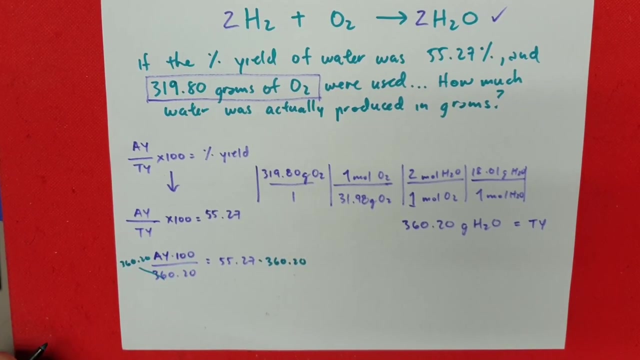 and I'm going to do that in another color so that it's a little bit more clear. so I multiply on both sides by 360.20 to cancel it out. so we have 55.27 times 360.20 gives us a big number. 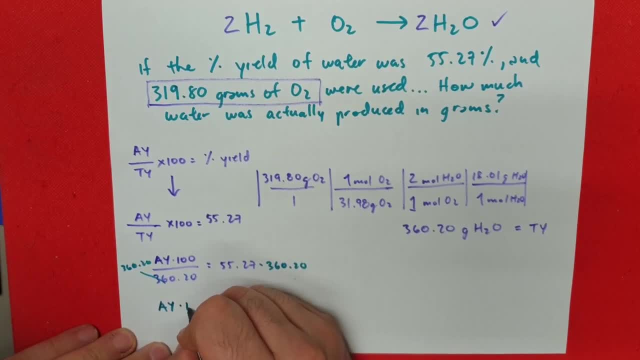 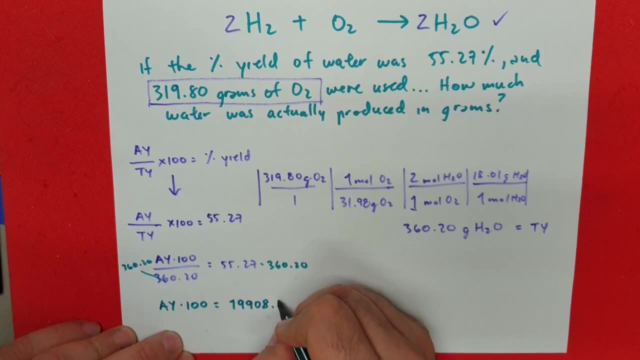 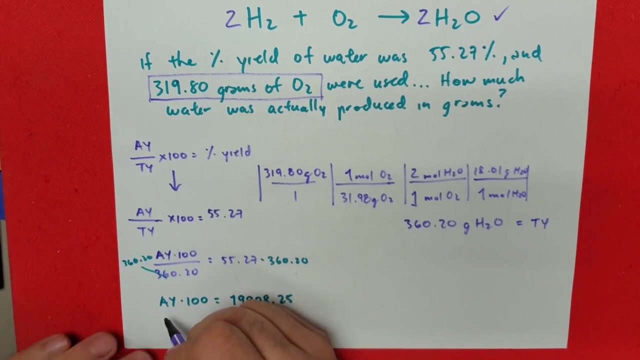 so we have the actual yield times: 100 is equal to 19,908.25 and at the end of the day we're going to take again the other marker and we're going to divide by 100 this time, and this is going to give us the actual yield. 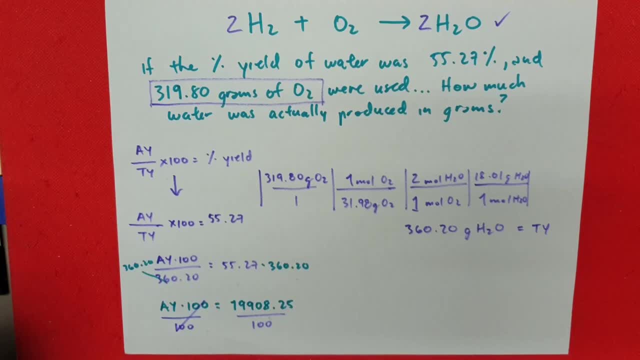 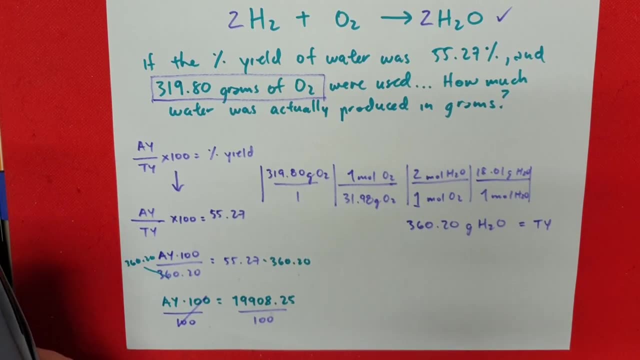 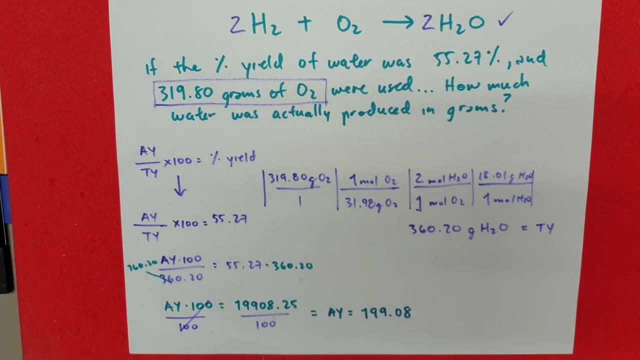 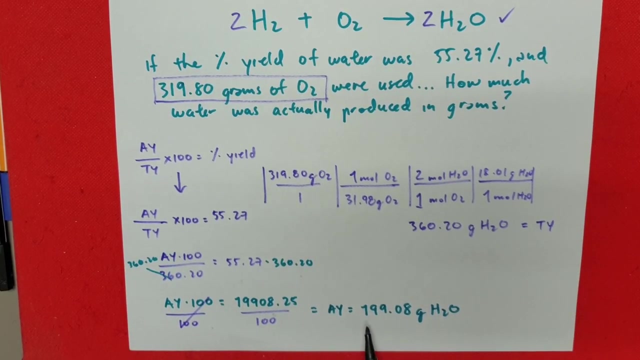 so we take 199.08 and we divide this by 100 and we have rounded up that the actual yield is 199.08 grams of water, which is what was being asked- grams of water. so we actually produced 199.08 when we should have produced, theoretically, 360. 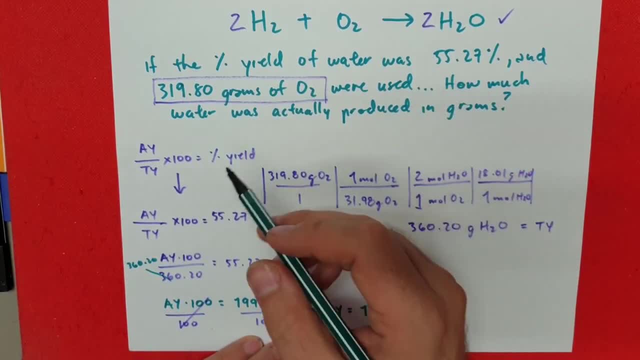 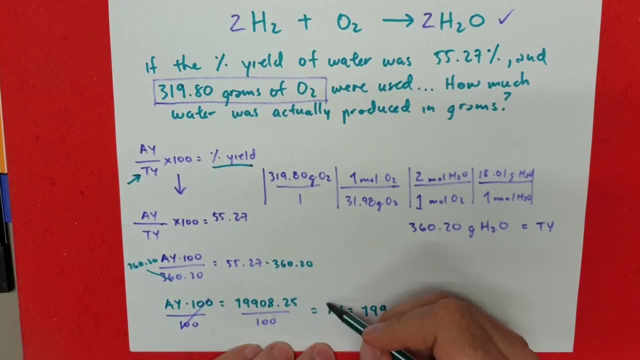 and we got this from the reverse exercise, where we were given the percent yield and we were given the percent yield and we were given the way to calculate theoretical yield. and then we did this, some algebra, and my actual yield of water is 199.08 grams. 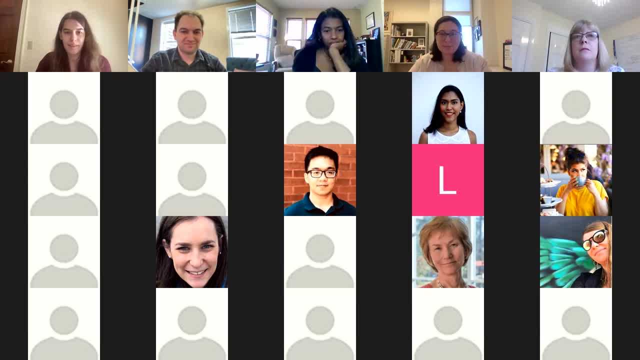 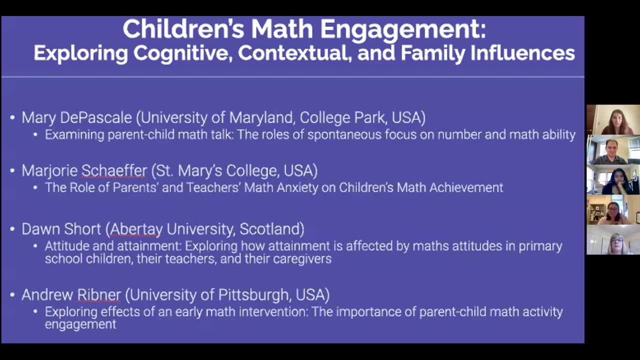 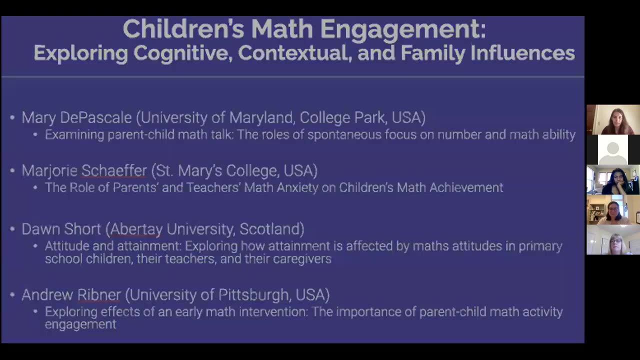 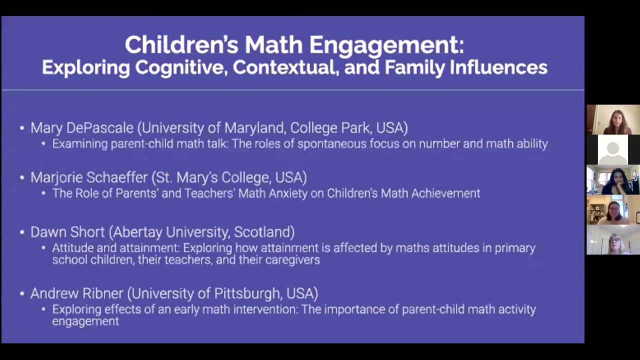 Our symposium is called Children's Math Engagement, Exploring Cognitive, Contextual and Family Influences, And so understanding influences on math engagement and math ability is important, And so our symposium has four talks that will examine factors that influence children's. 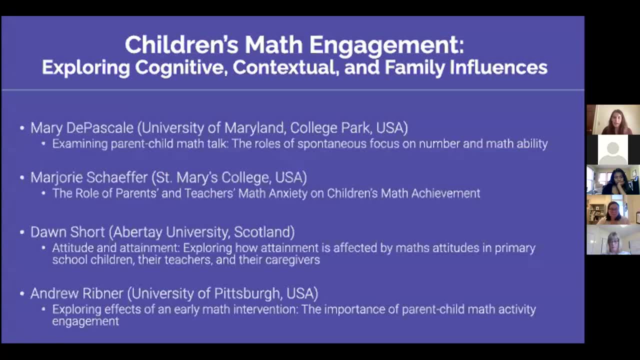 engagement in math, as well as the impact of engagement in math at home on children's math abilities. So first I will present on parent and child math talk and the role of spontaneous focus on number and math ability. Then, second, Marjorie Schaefer will present. 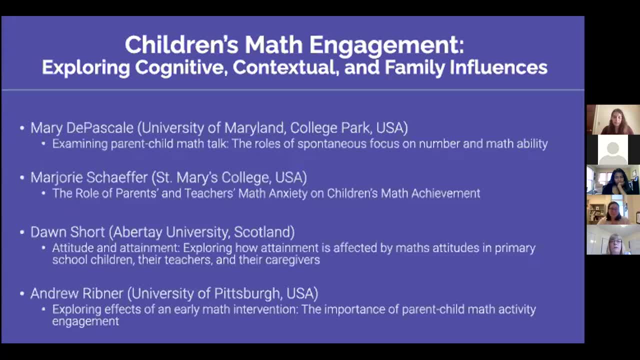 on the role of parents and teachers. math anxiety on children's math achievement. Third Dawn Short will present on how attainment is affected by math attitudes in children, teachers and caregivers. And finally, Andy Ribner will present on the effects of an early math intervention. 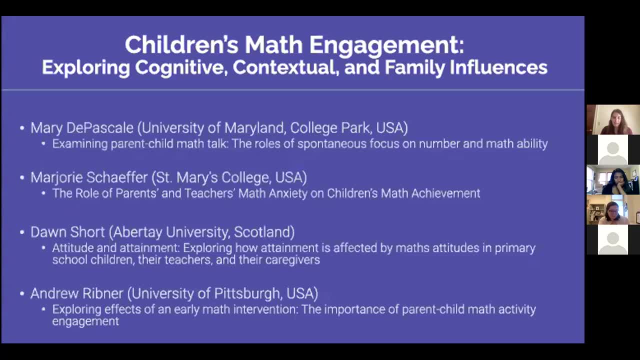 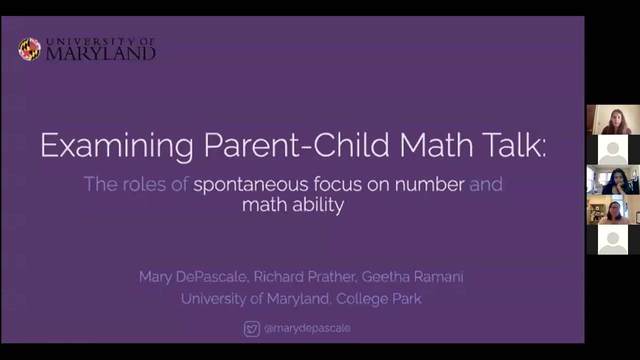 and parent-child math activity engagement, And we plan to have time for questions after each talk as well as at the end, if there's time, And Geetha and I will be monitoring the chat for questions as well. So I guess to start with my talk. So today I'll be. I'm going to start with my talk, So today I'll be.